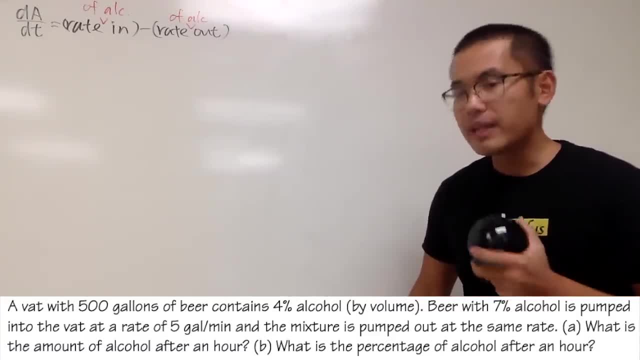 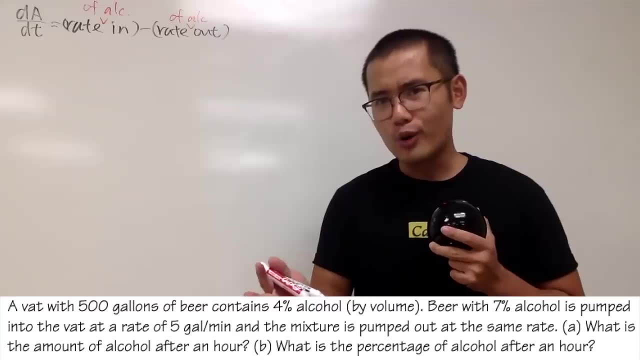 this case, right? Anyway, rate in minus, rate out. that's how you set up the differential equation, And the quick analogy is that suppose you make $300 per day but you spend $100 per day. So on your own, your rate of change of the money that you have is what? 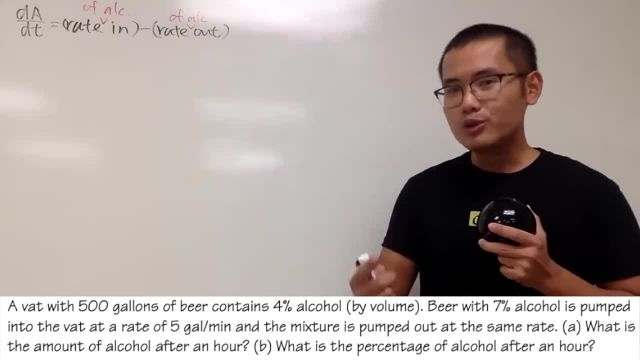 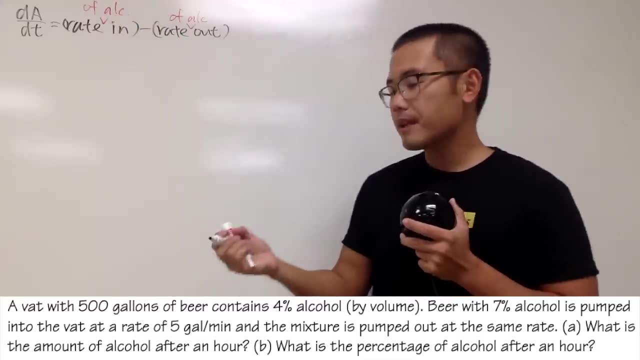 $200 per day, right? $300 in, $100 out, So it's $200.. Rate in minus, rate out And pay attention to one of the things that we're looking at for right. Okay, so to do this, we need two things. 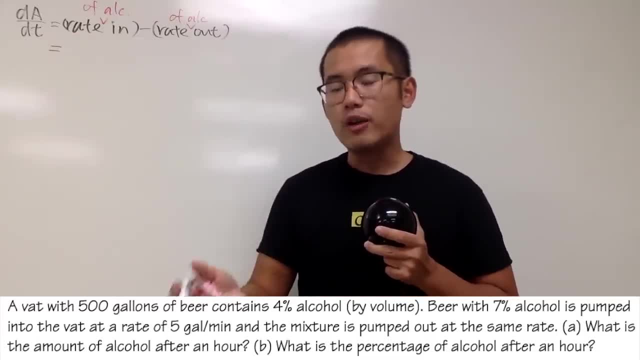 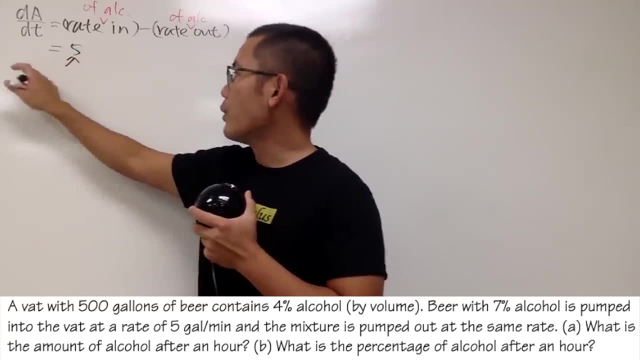 First of all, it says beer is coming into the tank at a rate of five gallons per minute. So let me put this down: This is five gallons per minute And this, right here, I will call it to be the flow-in rate. This is the flow-in rate, But this is not 100% alcohol. 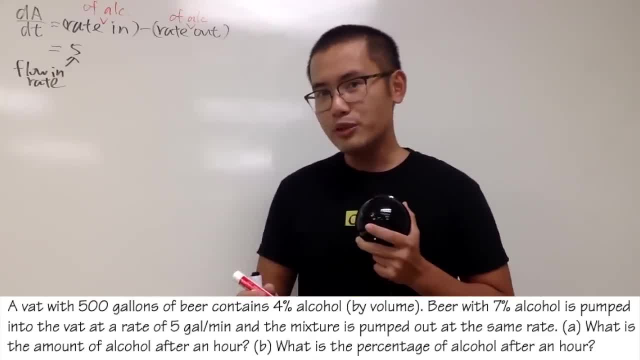 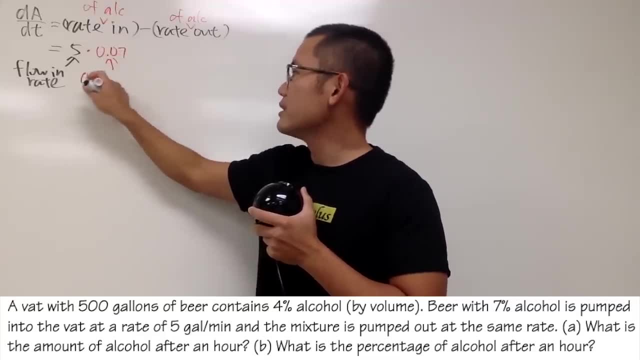 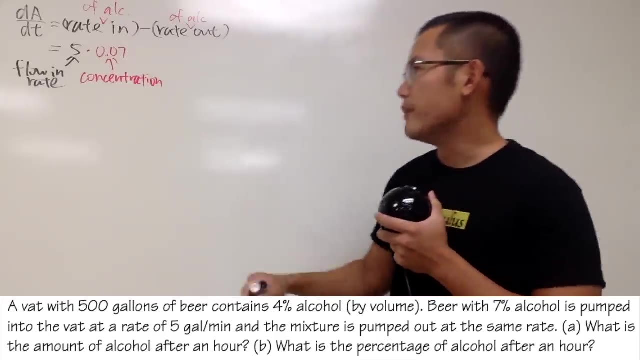 You have to pay attention to the concentration as well. And the concentration is what? 7%. Therefore, you multiply by 0.07.. And this, right here, is the concentration of the alcohol, right? So that's the idea. Technically, you just multiply it by the concentration of the alcohol. 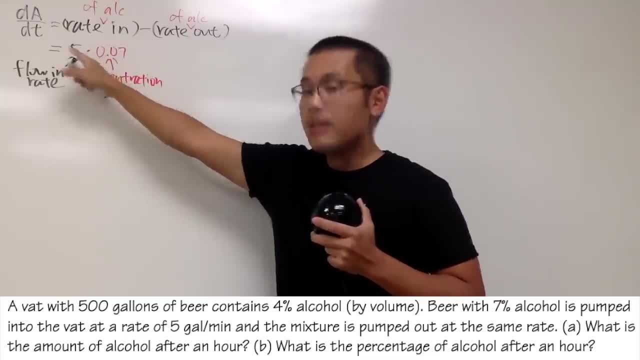 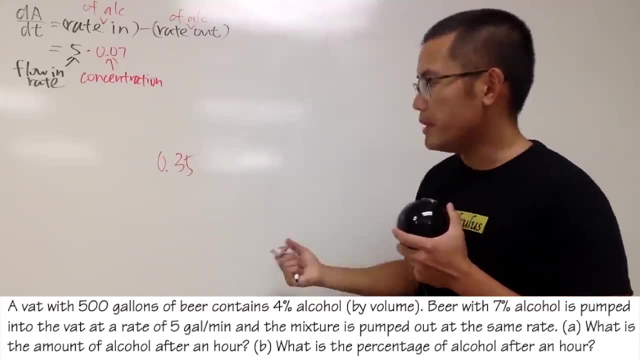 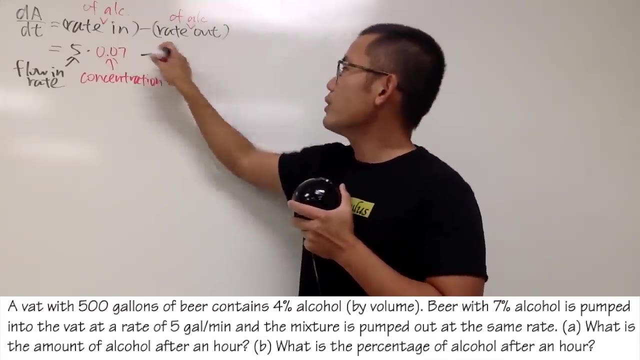 Multiply This is by gallon per minute times 0.07.. So it's 0.35 gallons of the actual alcohol per minute that's coming in, But we'll do this later. Set it out like this all the time, though. Next, we are also going to consider the flow-out rate, Because we're pumping out the beer at the 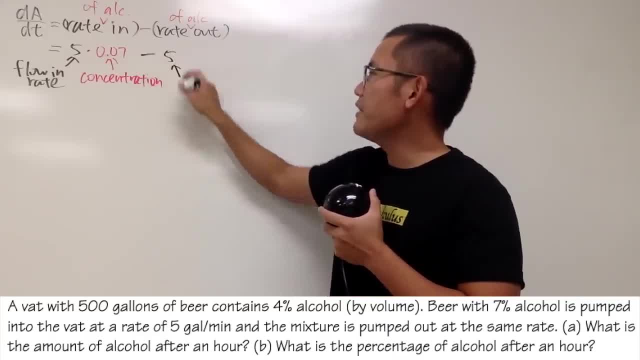 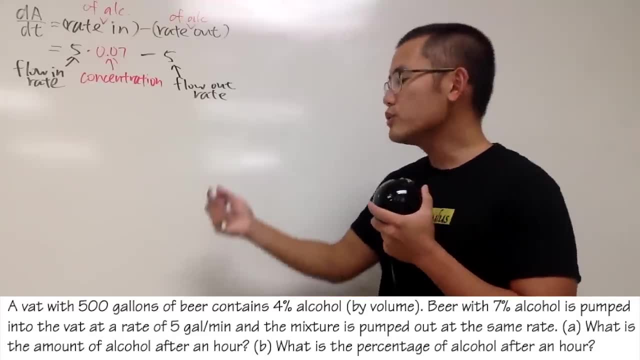 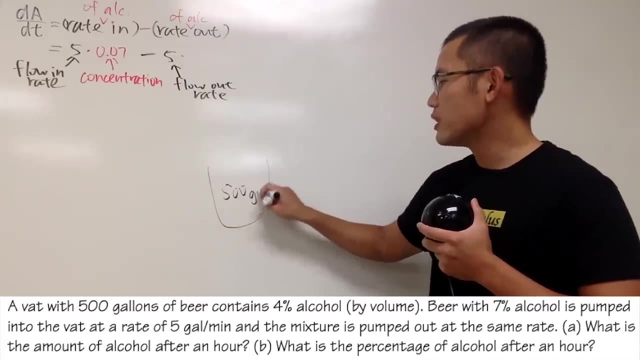 same rate, so it will still be five, And this five is the flow-out rate. Right, And now we also have to consider the concentration, though. Well, if you look at the vat, originally we have 500 gallons of beer. We have more coming in, but we are also draining out. 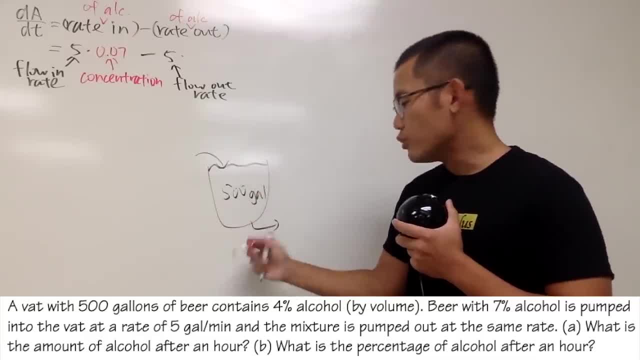 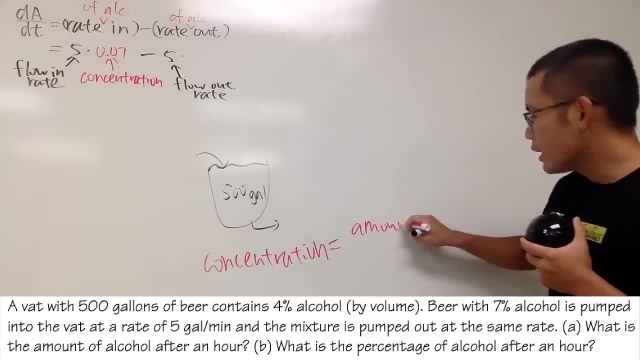 at the same rate. So the volume right here stays the same, And you have to remember that the concentration is what We need. two things to figure out: the concentration: The amount of whatever you are looking for divided by the total volume that you have. That's the idea. 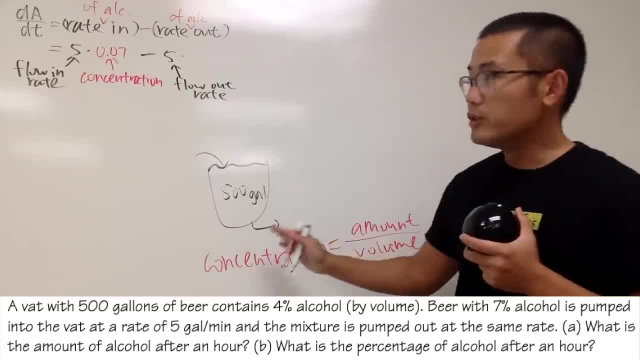 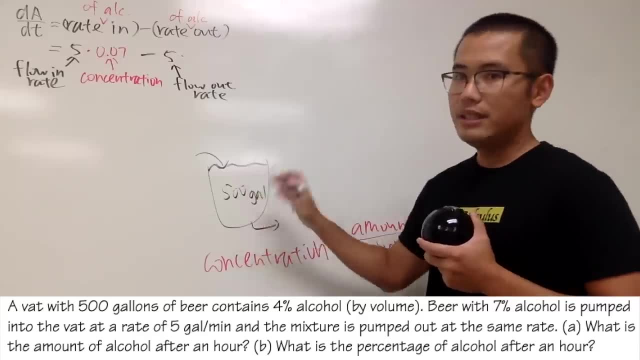 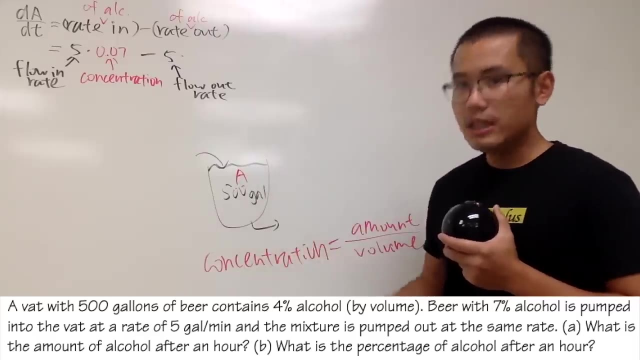 Well, keep in mind, originally you do have some alcohol already, but you have more coming in and some going out, Right, It changes in the vat And we already said that A is the amount of alcohol in this thing right here. So amount is just A. It's a variable, Right? So what you have to do is 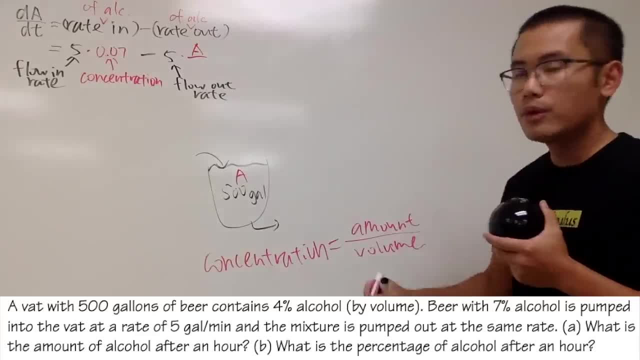 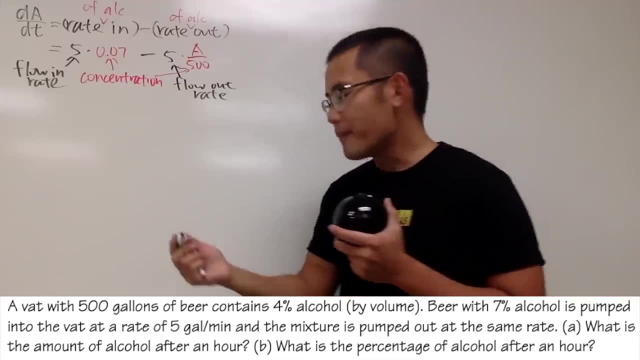 you actually do A and divide it by the volume, which is 500. This one, of course. So concentration right here. Yeah, All right, Now let's go ahead and put down what we know and what we want to know. We know this. 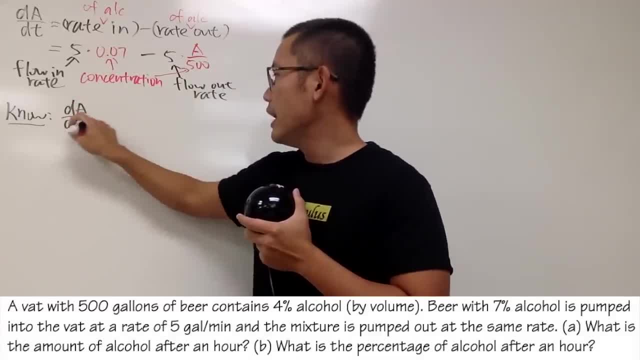 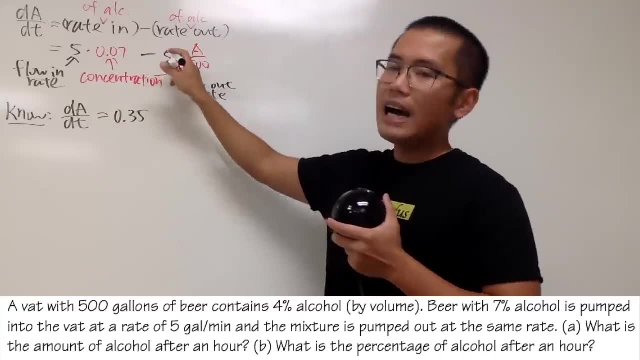 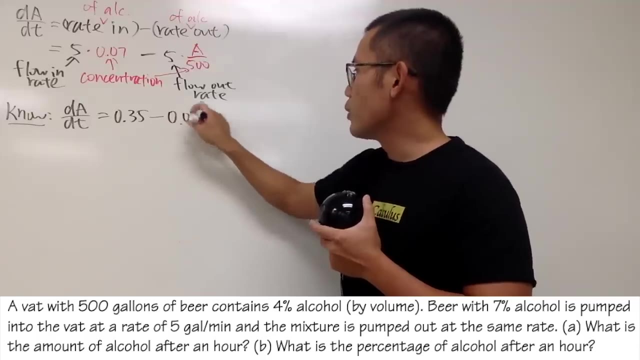 differential equation. So we have dA, dt, And now it's a good time to work this out. 5 times 0.07, that's 0.35.. And then 5 times 1 over 500.. Reduce it, You get 1 over 100, which is minus 0.01.. And 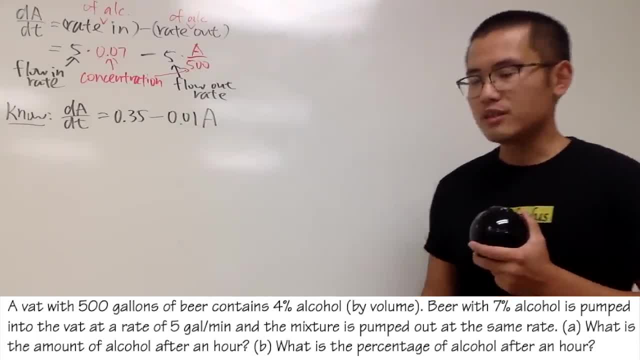 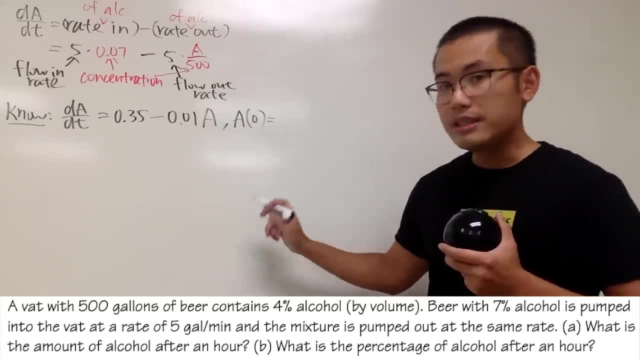 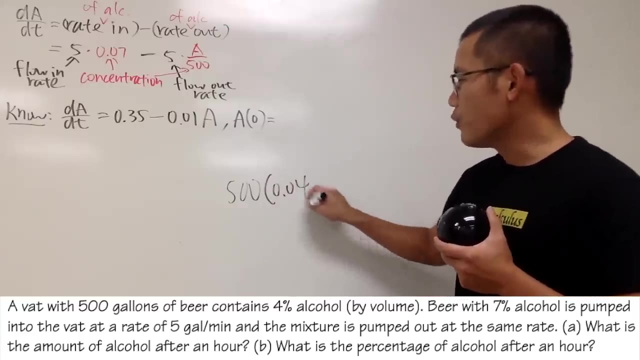 then you multiply by 8.. I find it easier if you just work with decimals, All right. And then we also going to see what's the initial amount of the alcohol that we have. Initially it says we have 500 gallon And only 4% of this is alcohol. So we have to multiply by 0.04.. And if you work this, 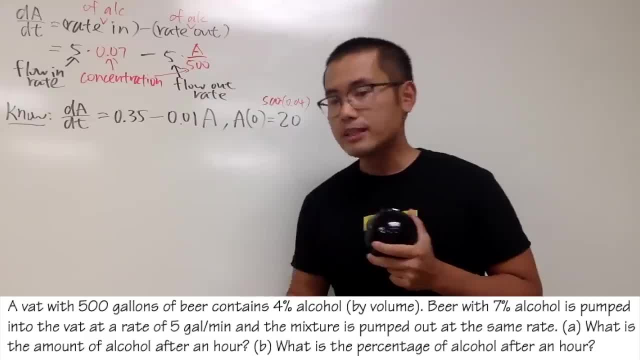 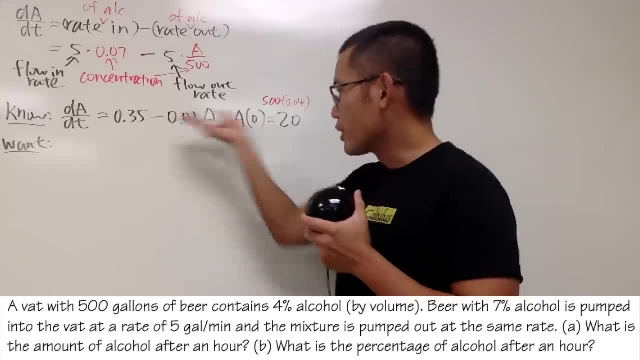 out, you will get 20.. So that's what we know. And now let's put down what we want to know. It says: we are trying to find out the amount of alcohol after one hour, But we are talking about minutes right here, So it will be A of 60.. Right, That's the amount of the alcohol after 60.. 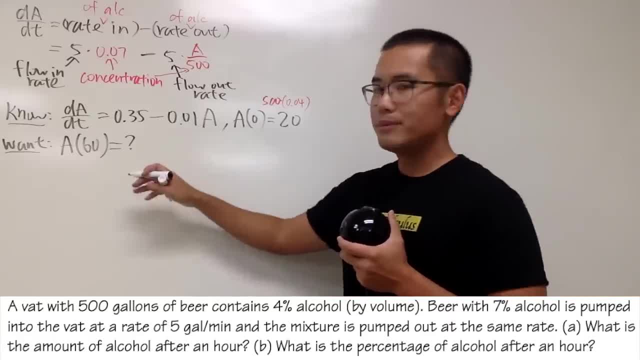 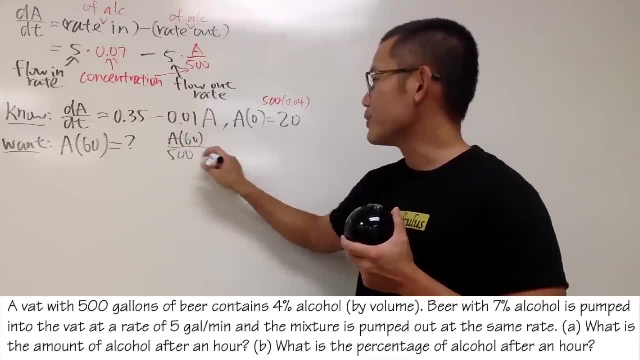 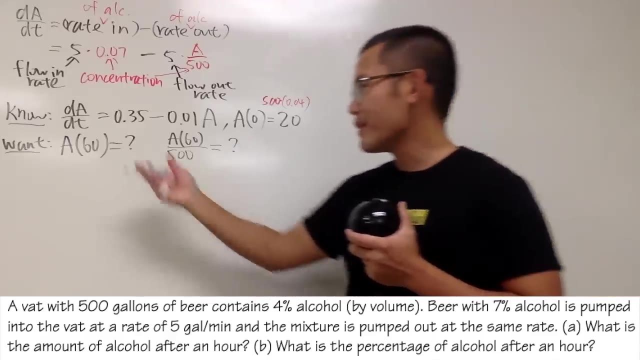 60 minutes And we also want to find out, well, the concentration of that. So we just have to do A of 60 divided by 500.. This, right here, will give us the concentration of the alcohol after one hour. So let's go ahead and solve the differential equation And then plug in 60. That's the idea. 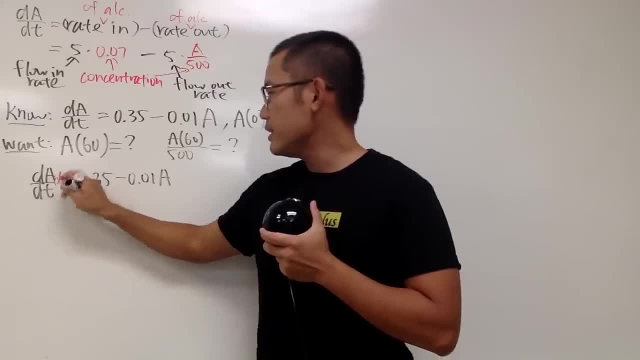 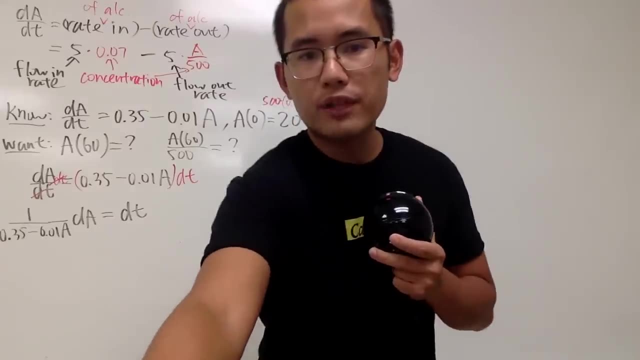 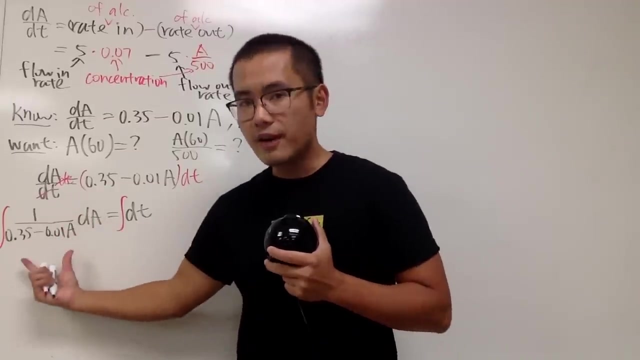 So here we go, And again, let's multiply dt on both sides, Put parentheses Right, And we'll also divide this on both sides, And then, once we separate the variables, we can of course integrate both sides. Here you see, we have 1 over linear function, So the integral of this. 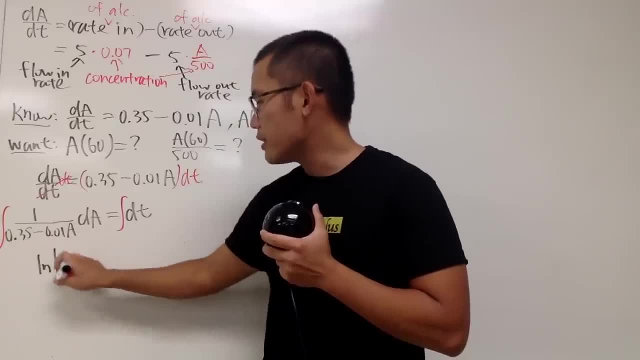 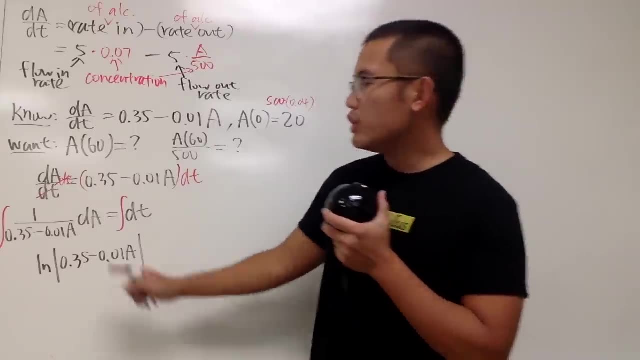 is just going to be natural log. absolute value of the denominator 0.35 minus 0.01A. But don't forget to divide it by the derivative of this. It's a number only You get negative 0.01.. Again, you have to divide it by that. 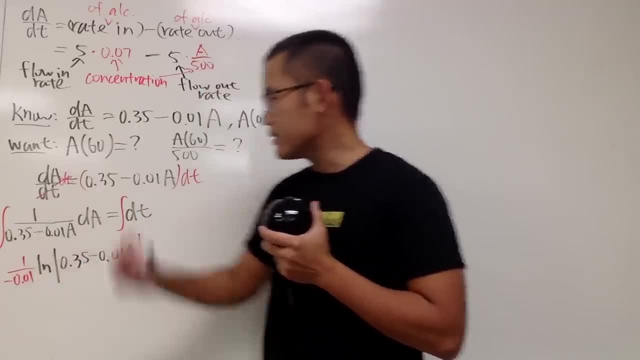 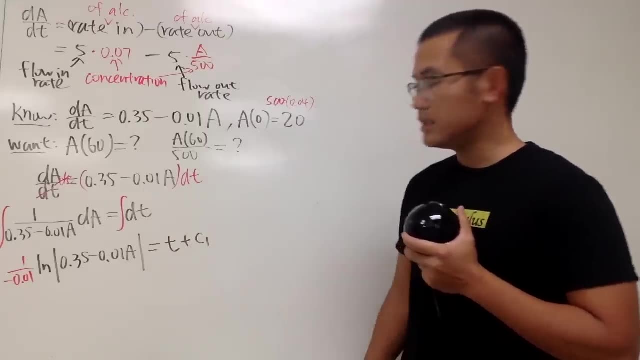 So I'll put it down as 1 over negative 0.01, like this. So that's it for the left-hand side. On the right-hand side, integrating this, we get t and then plus the first constant, C1.. 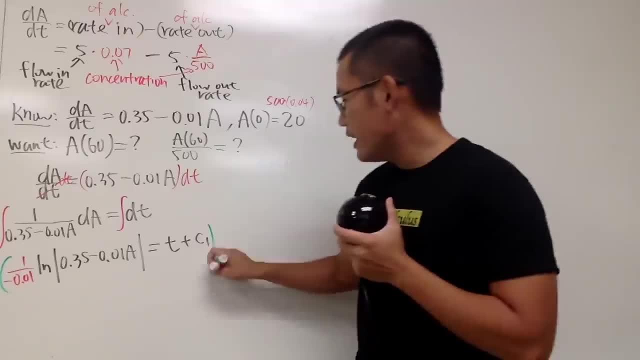 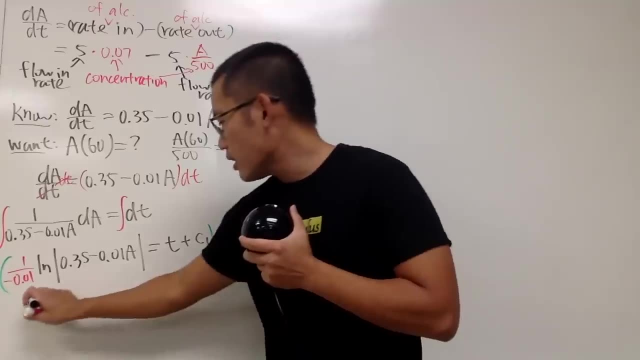 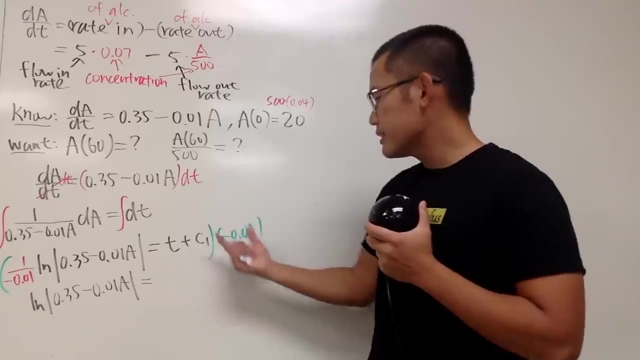 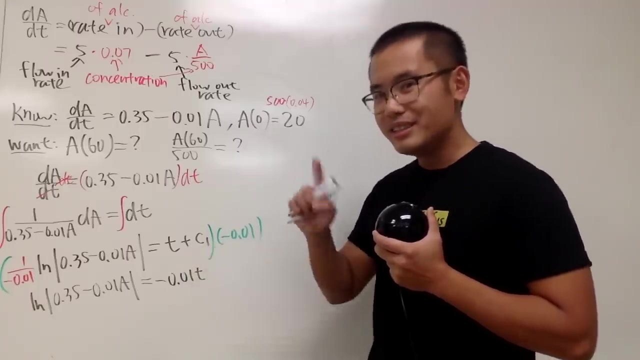 Now we just multiply both sides by negative 0.01.. So that this and that will cancel, And then we get natural log absolute value 0.35 minus 0.01A, And that's equal to this times that, Which is negative 0.01t. But this times that is just what C2.. So plus C2, right here. 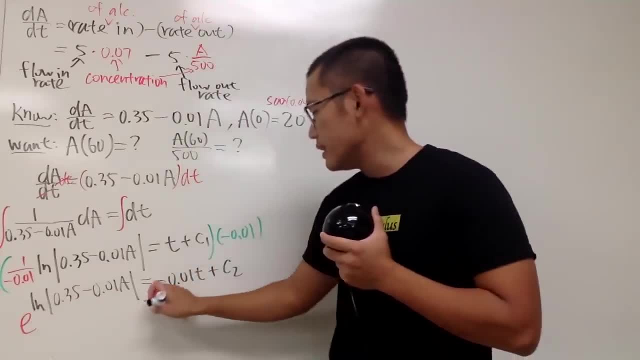 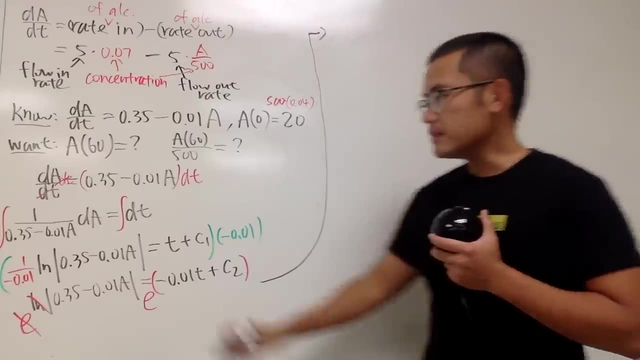 Now to get rid of the ln, we do e to this power and e to this power, And you see, this and that will cancel, And then, of course, we'll continue right here, On the left-hand side, we have the. 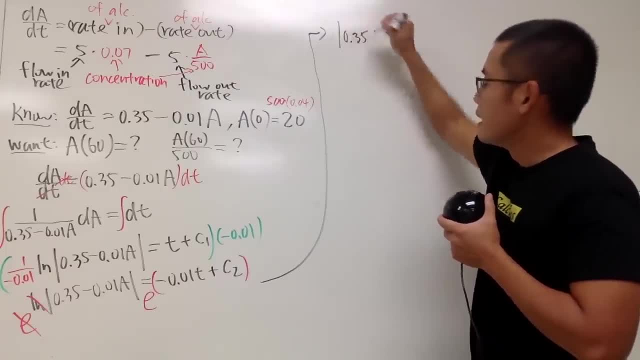 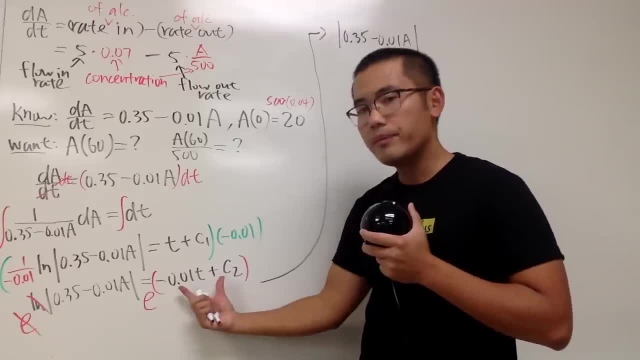 And that's equal to 0.01A, And that's equal to 0.01A, And that's equal to 0.01A, And that's equal to- here, the right-hand side, We have e to this power, which is the same as A. 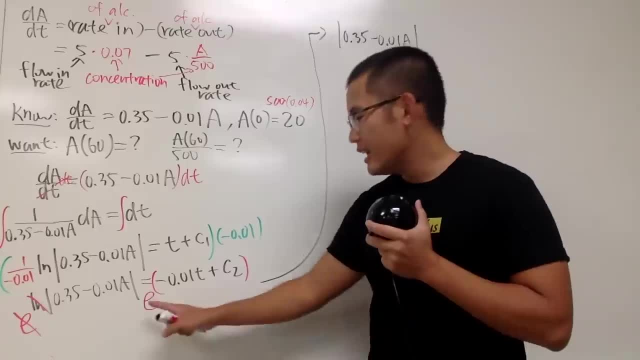 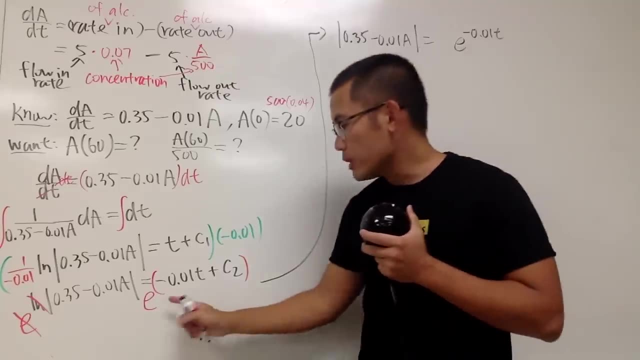 e to this power times e to that power. Let me write this down: which is e to the negative 0.01t, And then we multiply by e to the C2 power. But C2 is a constant, so it's e, So we can label that as. 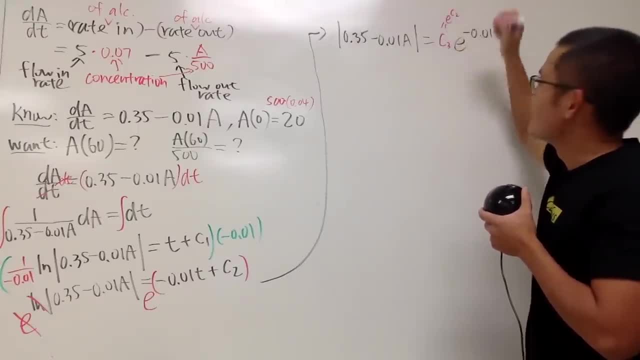 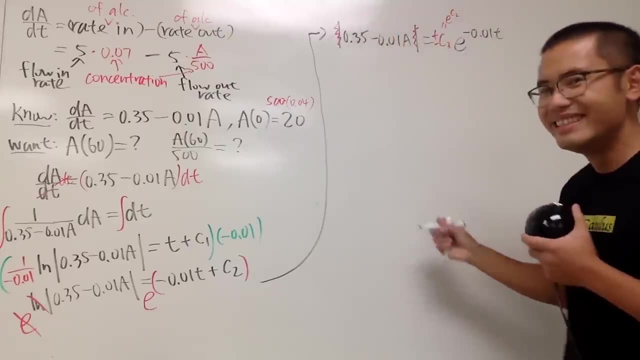 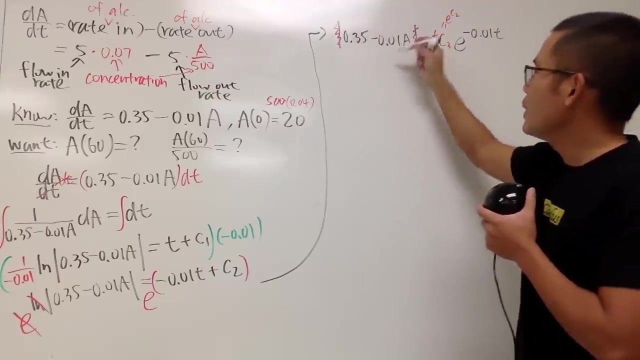 C3.. And again, this right here is e to the C2 power right Next, get rid of the absolute value, but don't forget to put a plus minus so we get this inside is equal to that, but let me also minus this on both sides, so we are looking at negative 0.01a. 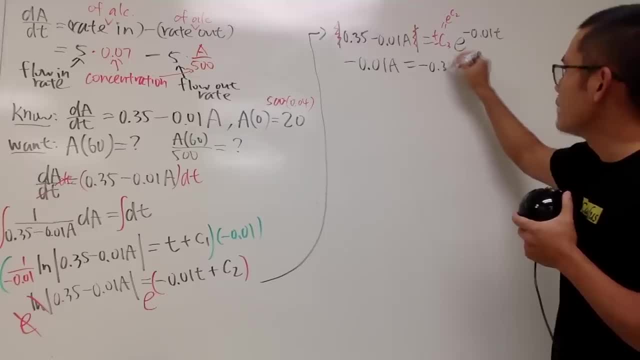 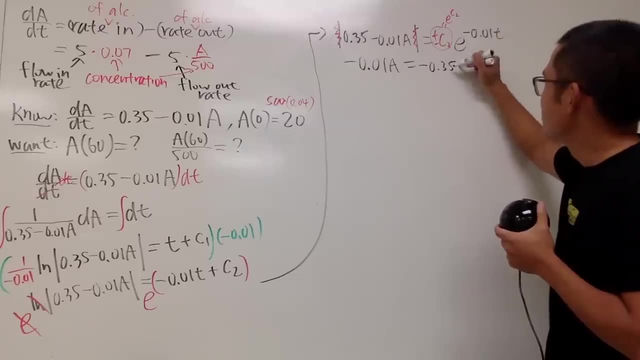 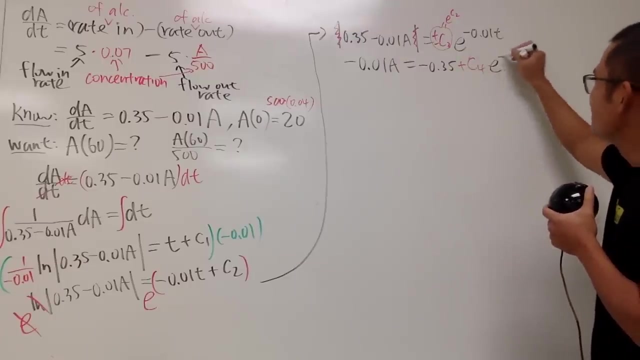 that's equal to negative 0.35,. here c3 is a constant, minus c3 is also a constant. so all in all, we'll put this down as plus c4, don't you have fun with that constant? and so does right. and then here we have e to the negative 0.01t, like this: 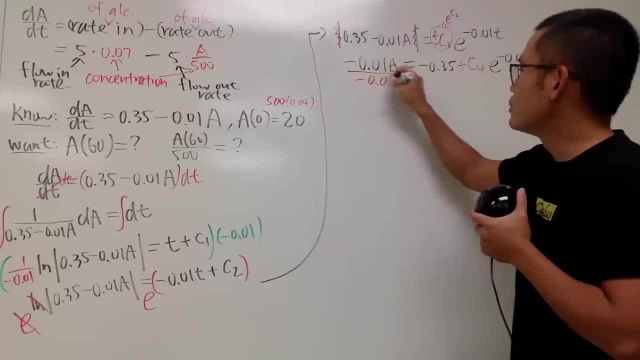 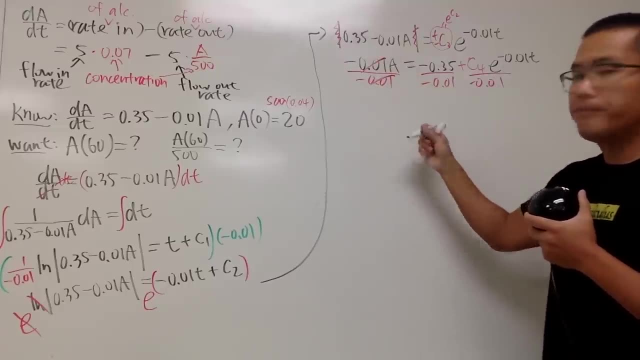 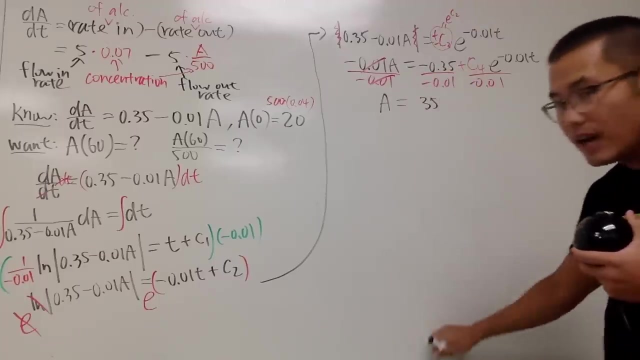 in the end, of course, divide everybody by negative 0.01,, divide everybody by negative 0.01, and all this right here, this and that cancel out nicely, and we just have a that's equal to well. this divided by that is positive 35,. now you see that. 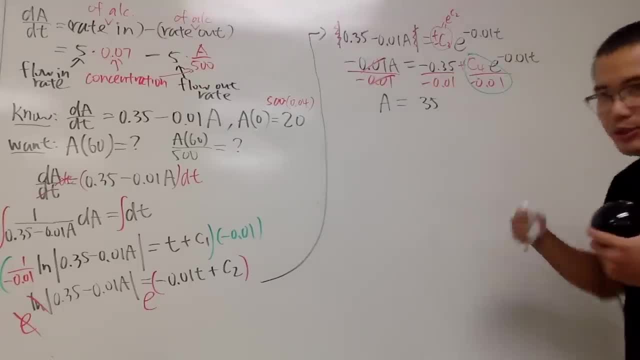 c4 is a constant, so is this? so this right here is just another constant, so you can legitimately put this down as what? just c5,? so put down c5 right here, and then e to the negative 0.01t. so that's pretty much how to solve this differential equation. 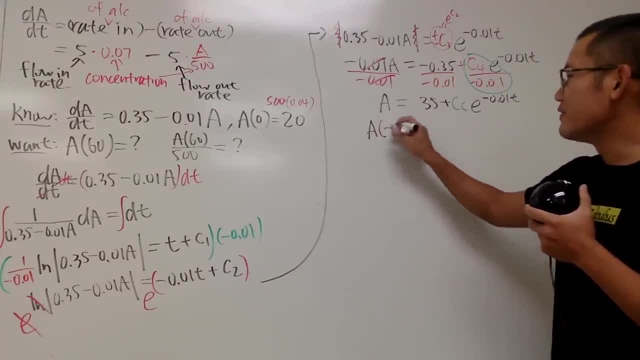 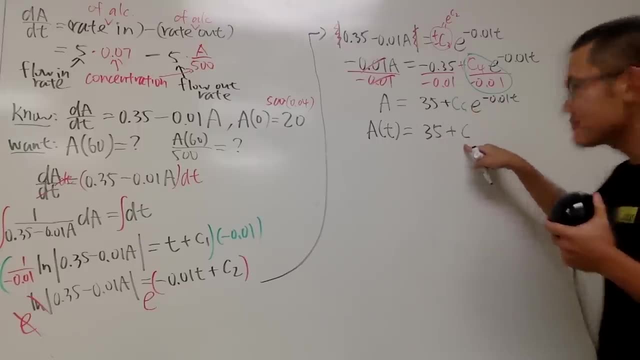 you are done. you know this right here represents a as a function of time, that's equal to 35, plus c- I'll just write it down c because we are done with the solving part, right, and this is e to the negative: 0.01t. 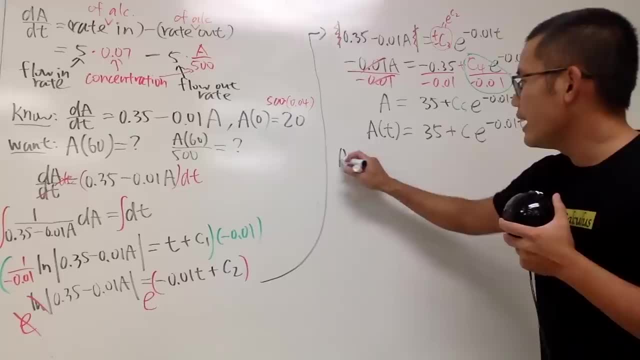 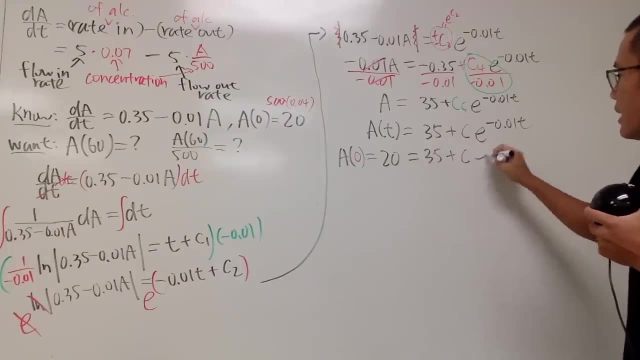 now, with this initial condition, we know a of 0, that will give us 20, and that means we have 35 plus c. e to the negative 0.01 times 0, will give us 20,. this right here is 0,, so e to the 0's power is 1, so we have 35 plus c equals 20,. 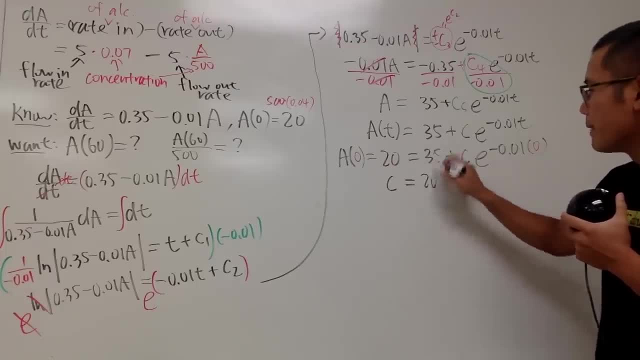 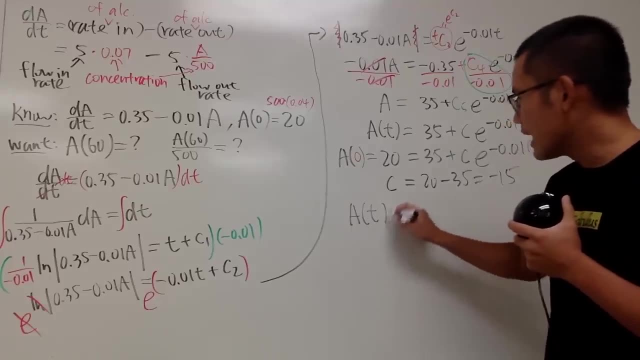 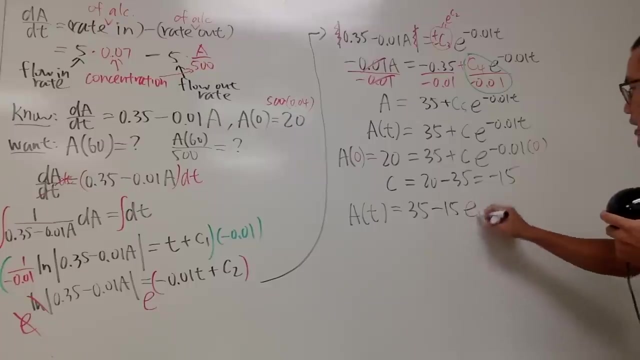 in another word, c is equal to 20 minus 35, which does negative 15, so we know a as a function of time is equal to 35 minus 15, and then we have this e to the negative 0.01t. 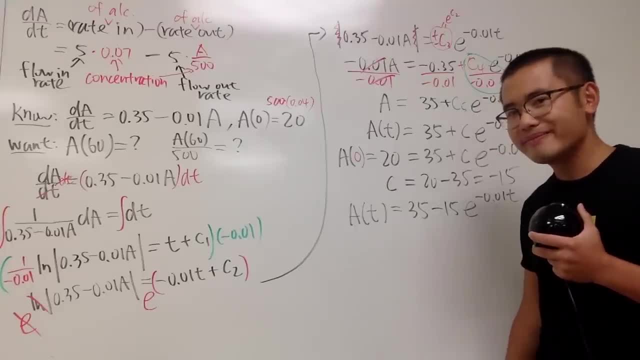 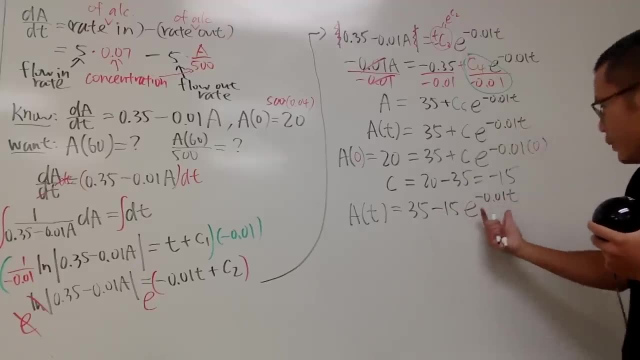 and check this out. is this an increasing function or decreasing function? Well, this part is a decreasing function, but this is a negative. a negative of a decreasing function is actually an increasing function. right, and you can see that this right. here it makes sense. 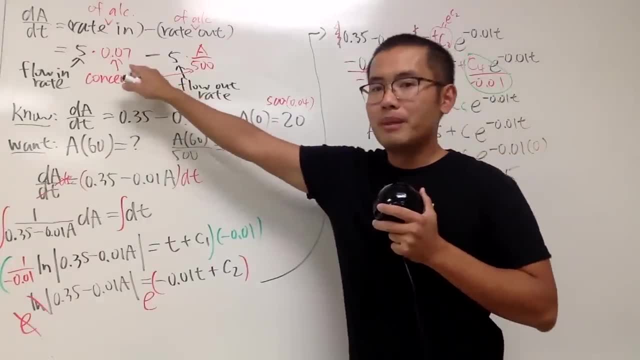 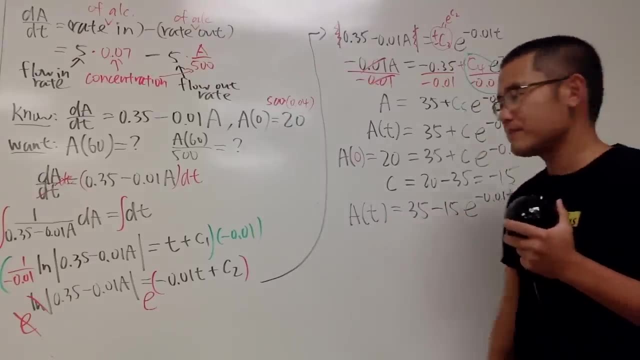 because you have 7% of the alcohol that's coming in is stronger than the original, which was only 4%. so the amount of alcohol in the tank should be more and there is a maximum, which is the 35 gallons of alcohol. 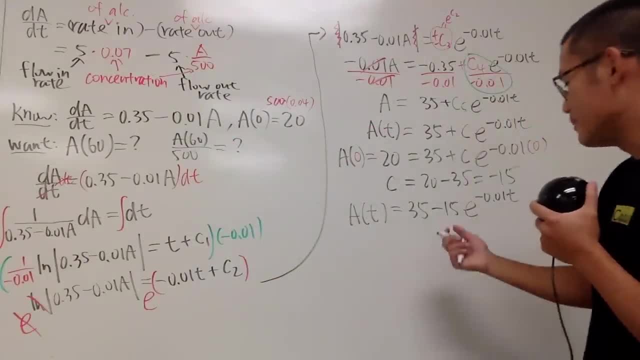 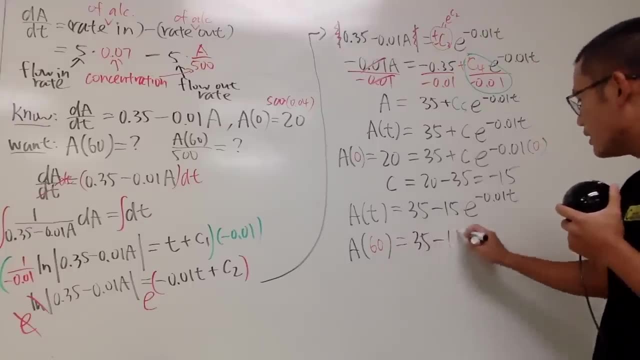 but anyway, let's figure out the a of 60 first, after 60 minutes. so here we go, a of 60, of course we can just plug in 60 into here and then use the calculator. that's about, oh so. 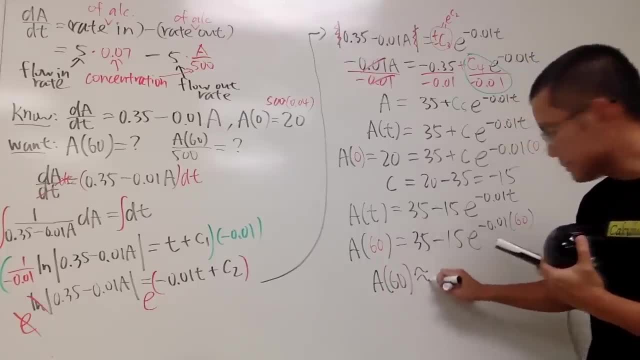 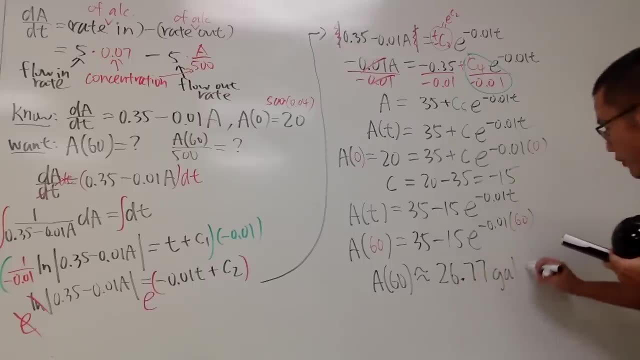 and we get a of 60,, it's approximately 26.77, and this is the number of gallons of the alcohol that we have right in the tank, right? so this, right here, is the first part. so here is the number of gallons of alcohol that we have. 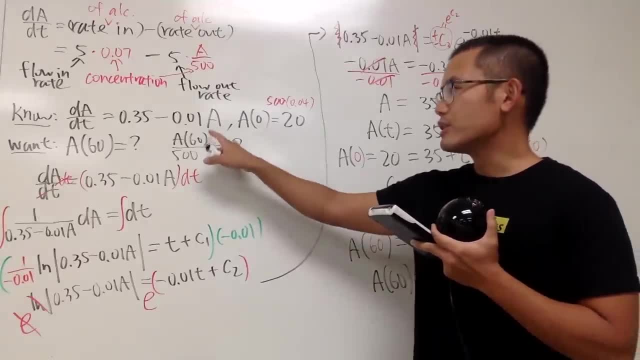 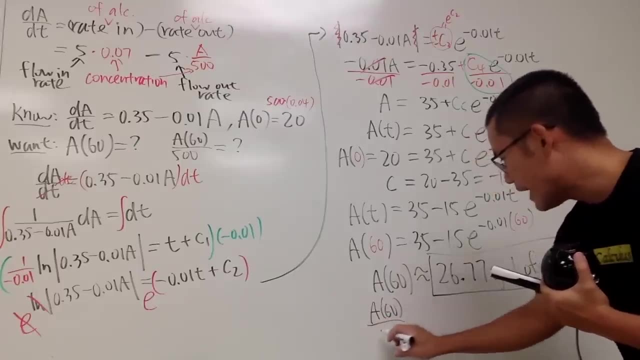 and the second part is that we also have to find out the concentration. so again, it's just the amount of the alcohol that we have divided by the volume. so if we do a of 60, divided by 500, so of course you just take this and divide it by 500,. 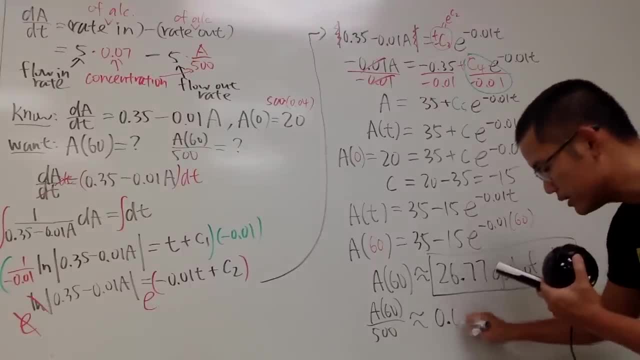 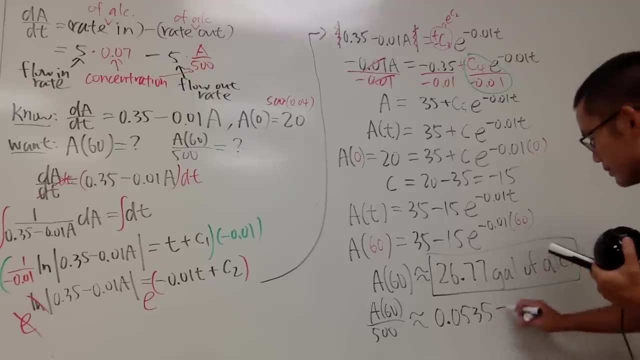 and you get approximately 0.0535, and of course that's the same as saying 5.35%. so this right here it's the percentage of the alcohol. so it's getting stronger and maybe just with another outward tool the beer will taste better. 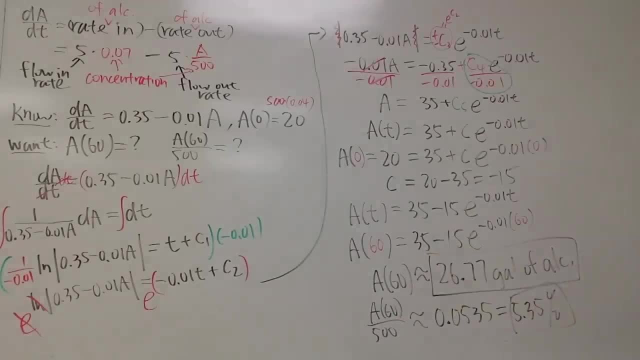 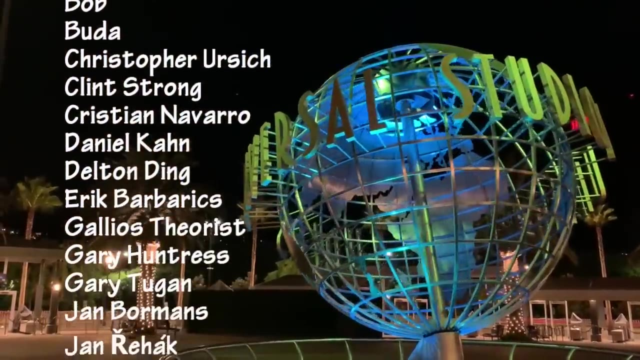 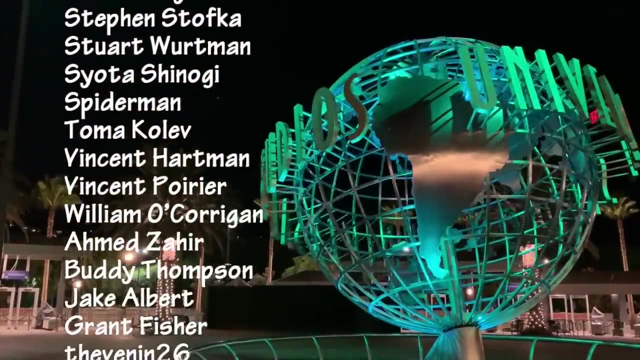 so anyway, that's the idea and hopefully this helps, right? ©? transcript: Emily Beynon. 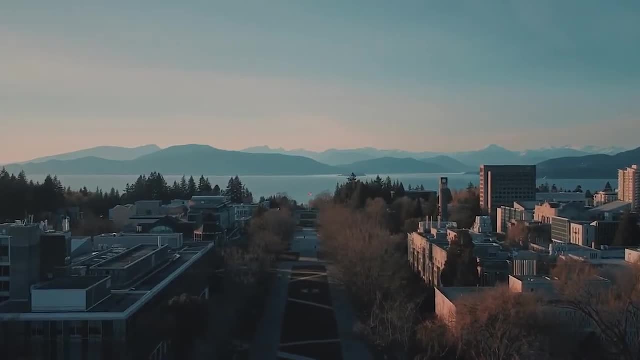 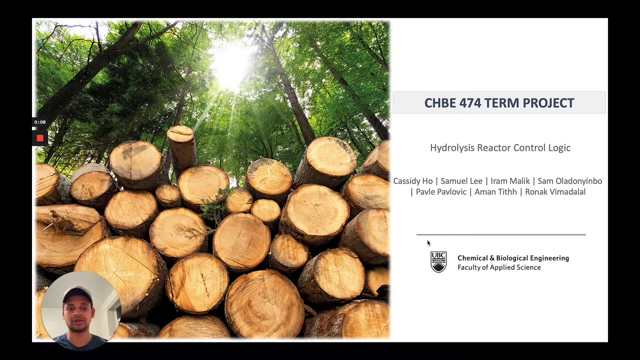 Hello professor, welcome to our presentation. Today we're going to be focusing on our process of extraction of hemicellulose from wood in a hydrolysis reactor, And in this presentation we'll focus on the entire control strategy that goes towards implementing this process.